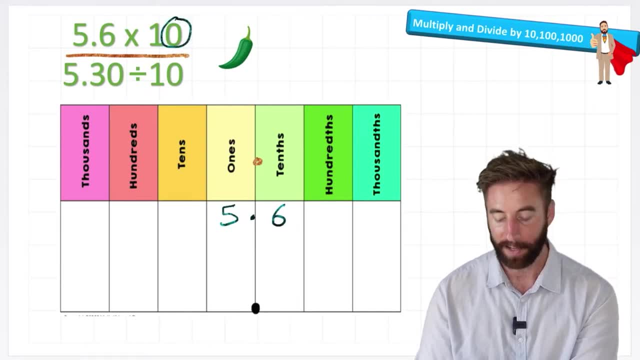 little hint with that, because we have one zero in 10.. And which way are we going to move? Well, we know we're going to be moving up the place value chart To the left because we're getting a larger value timesing. So here we go, Let's start. I'm going to 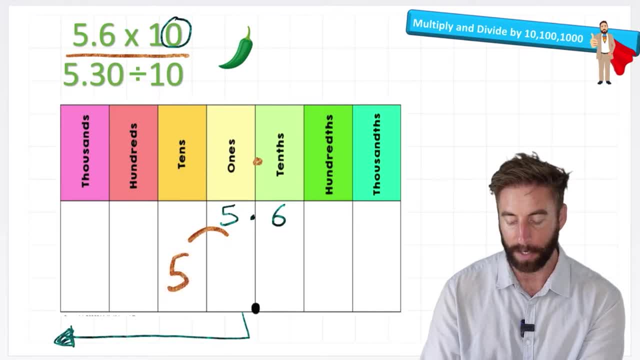 move my five one position here. I'm going to move my six one position here And I'm going to put my decimal point back, just for the sake of it. So now I can see that my answer to 5.6 times 10 equals. 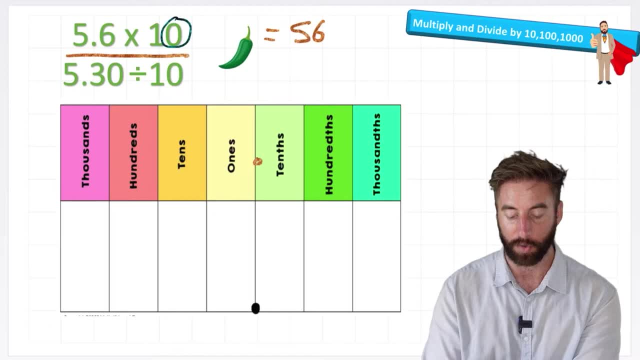 56.. Okay, and let's look how it can help us with division as well. So my next question says 5.30 divided by 10.. So the first thing to do is put our numbers in the correct place. 5.30 is five ones, my decimal three tenths and zero hundredths, And again we're dividing by 10.. So 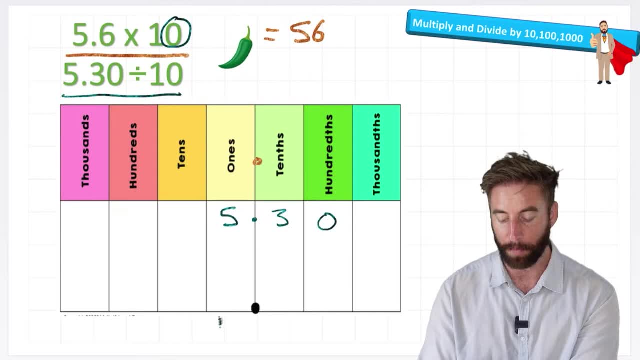 I'm only going to be moving one place, But this time I'm actually going to be moving my digits down the place value chart because I'm dividing, so therefore my answers are going to be getting smaller. So here we go, Let's move them one place. My five now comes into the 10th column. My three: 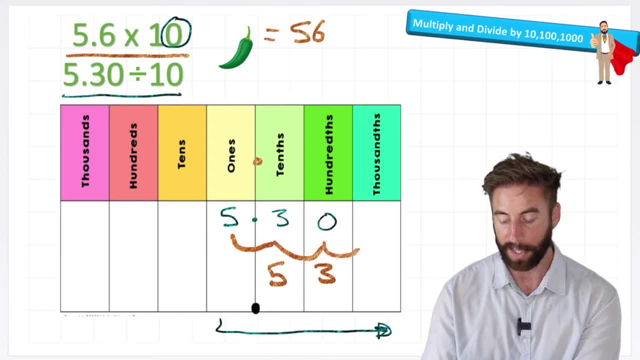 goes into the hundreds column and my zero goes into the thousandths column. But now I need to put my decimal back And I have a choice: I can either put a zero here or I could leave it without. But either way my value doesn't change. My answer is 0.530 or 0.530. And again. 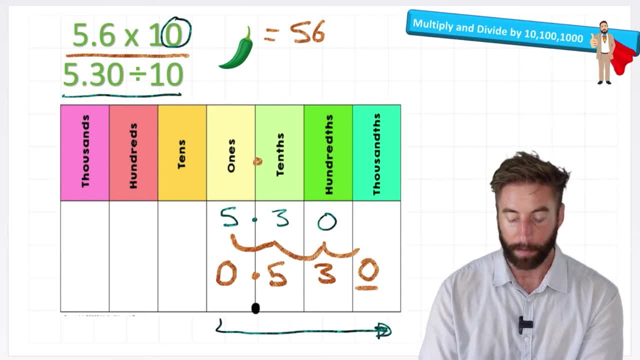 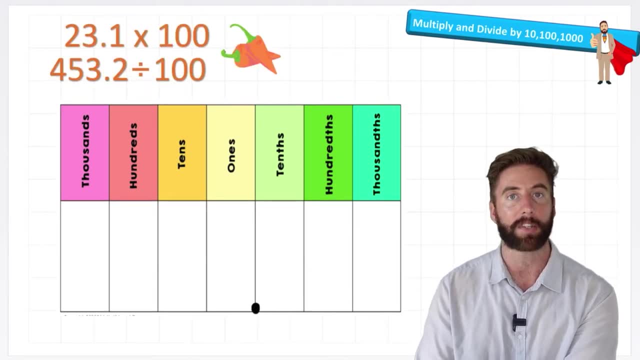 this little zero at the end. we actually don't need. it doesn't change the value. So my answer, in its simplest form, is 0.53.. Okay, let's get a little harder. We're going to look at timesing and dividing. 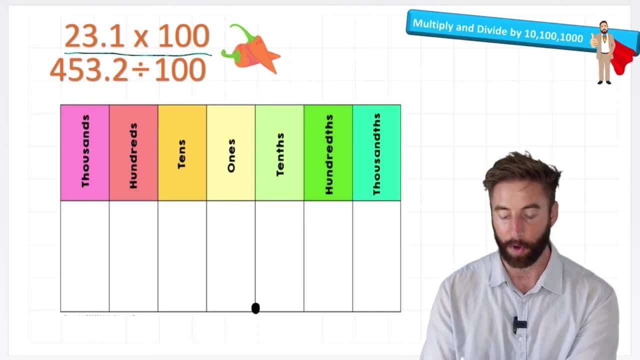 by 100.. 0.53.1 times 100.. First things first, again put our number in the correct place, And this time I'm timesing by 100.. So I now need to think about moving my digits, not one, but two places up my. 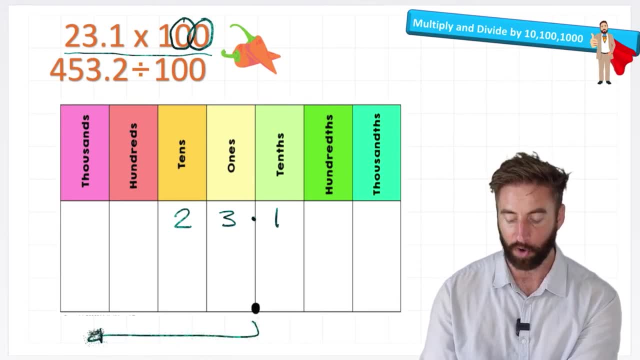 place value chart. So again we're coming left or greater up the place value chart, but I'm going to move them two times. Here we go: My two goes one two, my three comes one two And my one one two. But now I have this gap before the decimal And I need to fill this gap. 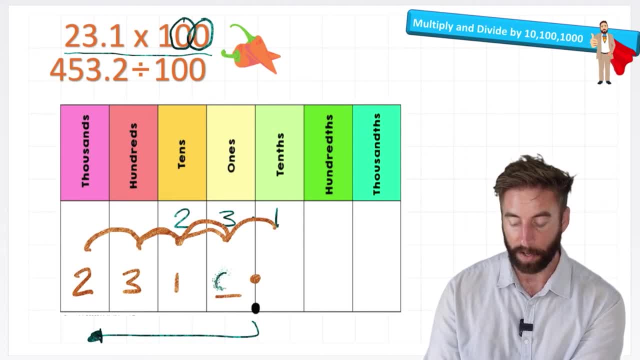 Otherwise I won't have a complete number, So I'm going to fill it with a placeholder or a zero. Therefore, my answer to 23.1 times 100 equals 2310.. Okay, next is my division. I have 453.2.. There we. 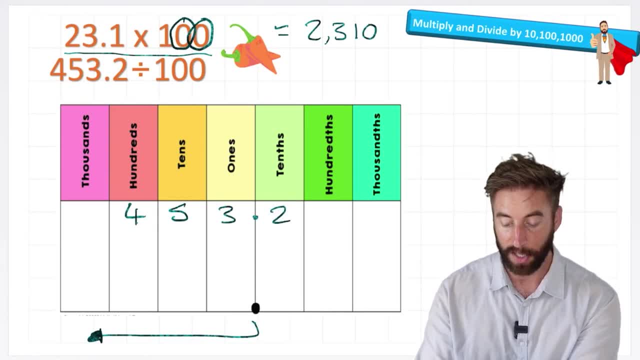 go all ready to begin And I'm dividing by 100.. So this time I'm not going to move up the place value chart. I'm actually going to be moving down the place value chart. So how many times am I moving again? one, two zeros in my 100. Or a different way of thinking about it: 100 times. 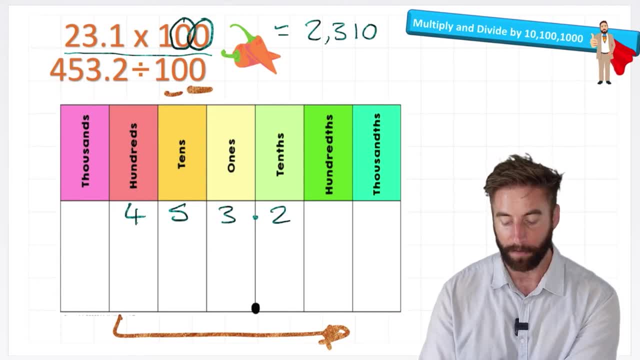 greater is going to be two columns across, So I'm gonna start with my four, move it one two, then my five, one two. my three: one two and my two, one two. Very important, I don't forget to put my 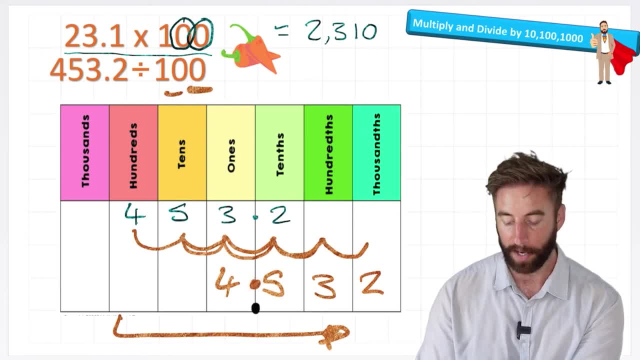 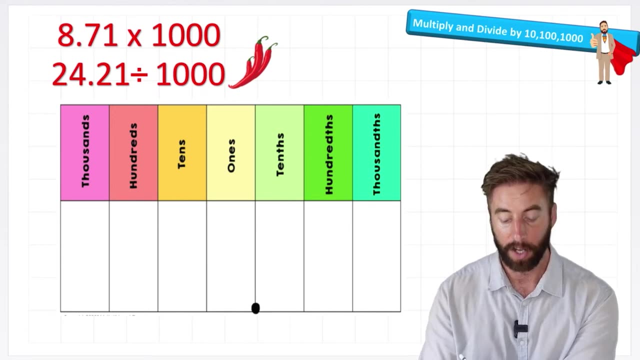 decimal. back at this point. My decimal always stays on the decimal line. So my answer to 453.2 divided by 100 equals 4.532.. Nice, let's start our hardest ones. then we have timesing and dividing by 1000.. First question says: 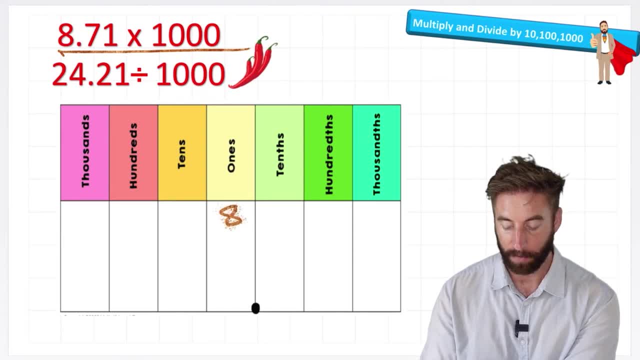 8.71 times 1000. So I'm going to put my 8.71 in the correct places And now I'm timesing by 1000. So hopefully we've caught on to the pattern. Once again we've got 123 zeros in our 1000. So I'm going to be moving them one, two, three places. 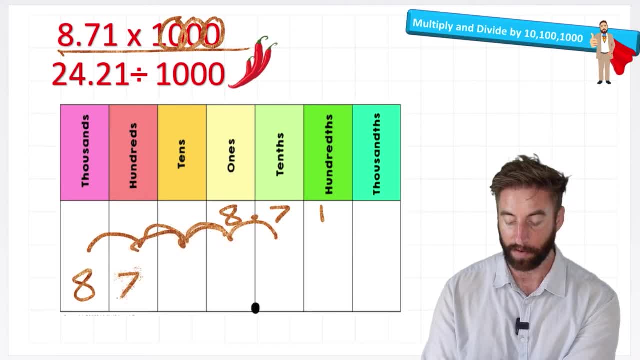 do the same to the seven: one, two, three. to the same to the one: one, two, three. And again, just like before, we have this blank column before the decimal, so we need to fill that in And we're. 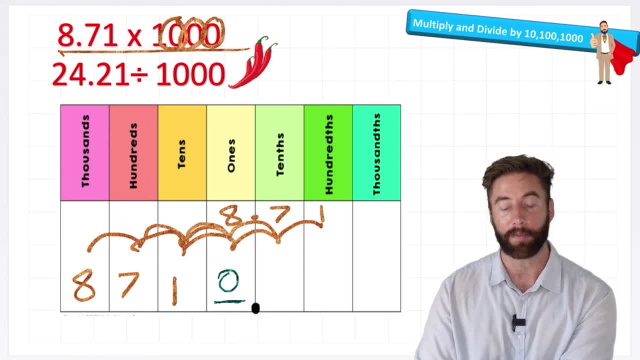 going to fill it with a placeholder. So my answer to 8.71 times 1000 equals 8710.. Chapman Zwei: 1 to 10蛋 and 0 has a zero as we get to Friedman L. 1 to 10蛋 has a zero as we get to Friedman L. 11 to 10蛋 tand和a 0 pel. 거기 weுd 150 times 0 Parliament onlineungluing力. 1 to 10蛋和a 0.1 Auntie. we're moving at 0 По.1 in our 1000.. So I'm just going to keep that one. the 2 places which 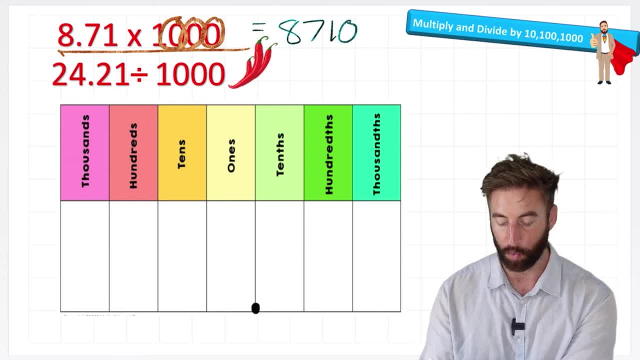 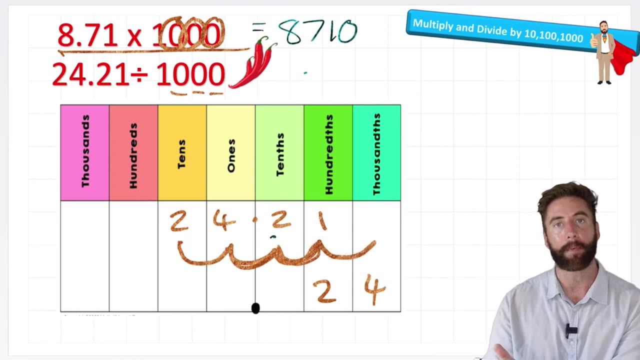 and 10. last but not least, 24.21 divided by a thousand. and again we're moving one, two, three places. so let's begin. i have my two moving one, two, three. my four will also go. one, two, three. okay, but before i can move this two, i can see already that i'm not going to have a column to 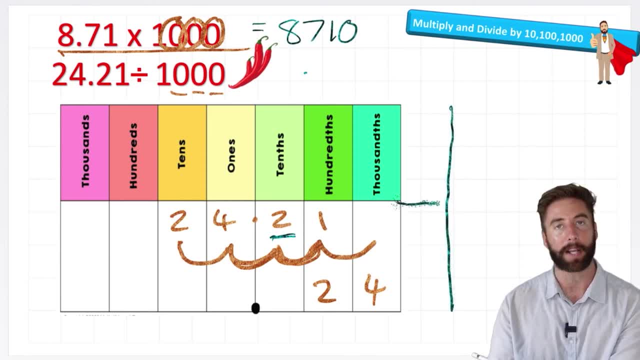 move it into. so i'm going to create a new column because, remember our place value charts can go on indefinitely in either direction, and this will become the ten thousands column, and i think i'm going to need another one for the one that's next to it. so i add another one as well, and this will 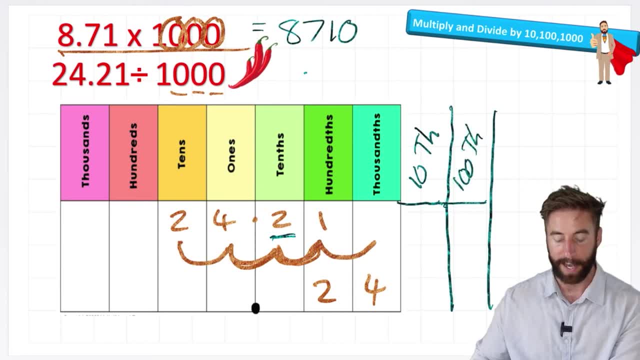 become the hundred thousand column. now i can carry on. i'll move my two, one, two, three places into the ten thousand and my one, one, two, three places into the hundred thousands. but again i can see a small gap here, next to my decimal, which i must fill with a placeholder. so my answer to 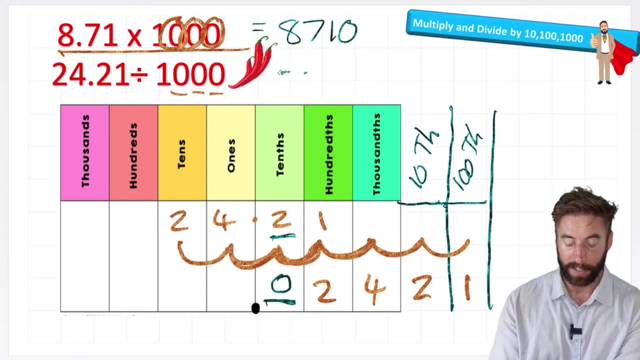 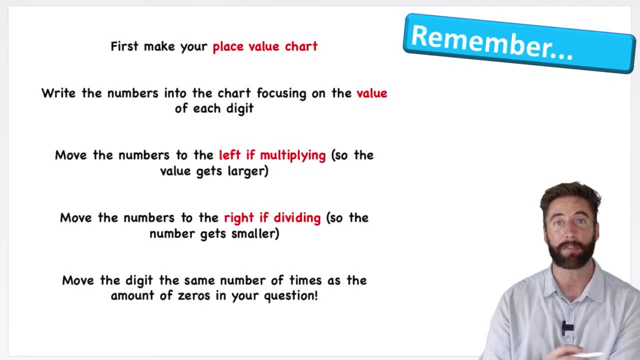 24.2. one divided by a thousand is 0.2421. and there we have it. that is everything you need to know about timesing and dividing decimals by 10, 100 or even a thousand. things to remember: always start with your place value chart when you're writing the numbers, in focus on the value of each of the 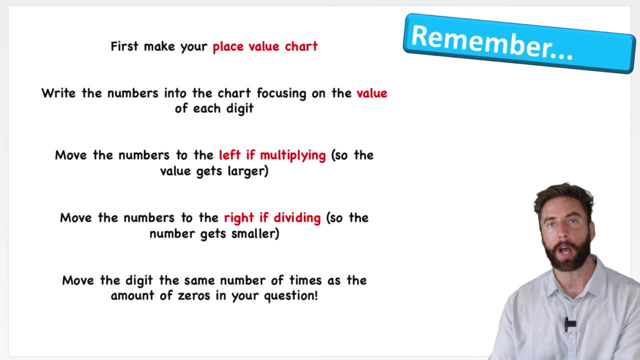 digits to make sure you put them in the right column. and remember that when we multiply and we move up the place value chart to our left and when we're dividing we move down the place value chart to our right. to know how many columns we're going to move our number, we can simply 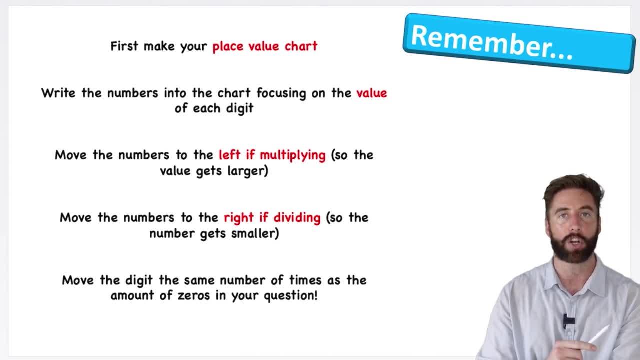 look at our question and if we're multiplying by 10, that is only one position: 100 2, 1003, and that number corresponds to the amount of zeros that are in the question. okay, so here are a few questions for you to work on. build your own place value chart and put your answers in the comment. 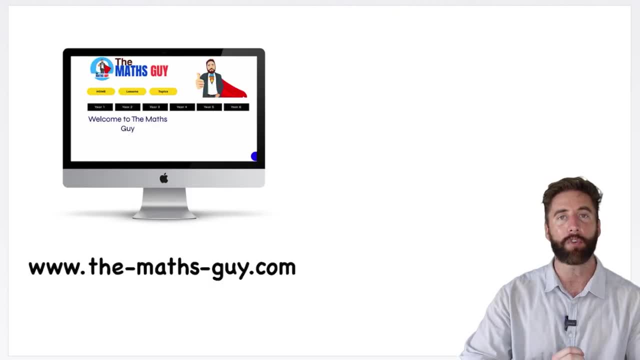 section. i'm going to mark them all. okay, hopefully this video has been helpful for you. if it has, subscribe to the channel, but for now, peace out.